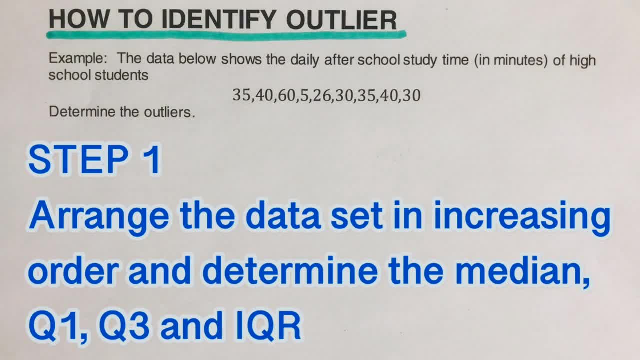 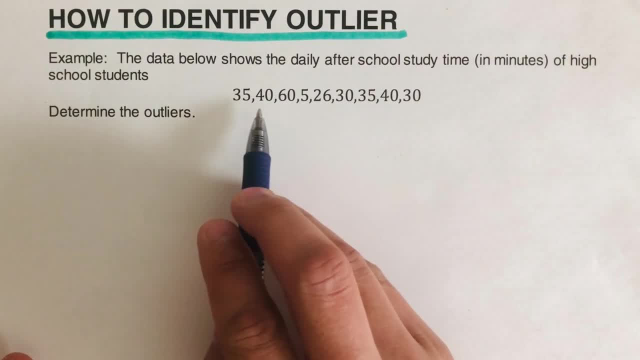 we determine the median, first quartile, Q1,, third quartile, Q3, and the IQR. So, going through this problem that we have here, we are supposed to determine the outlier. So let's take this first example right here. Let's tell our student that ID had to be outlier by partly That students 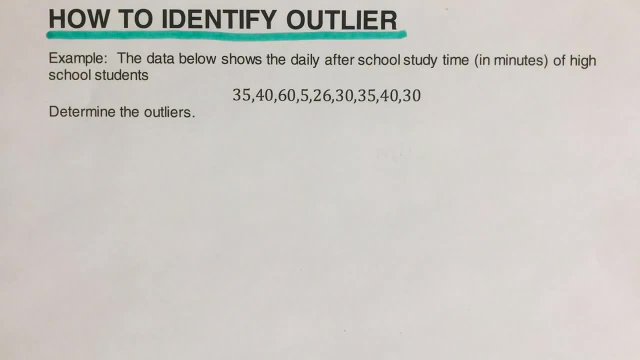 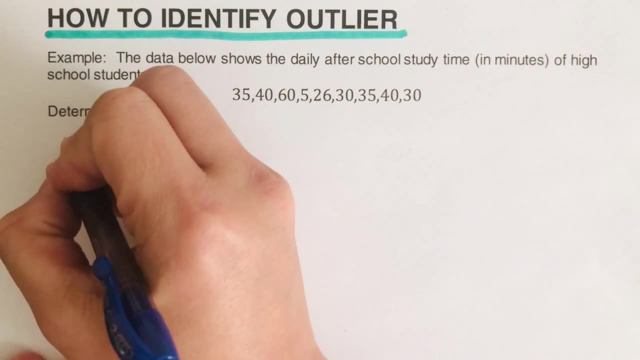 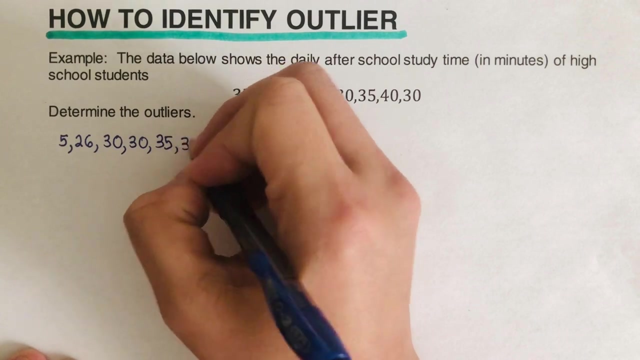 say that this, I guess, is not true. So I suggested to arrange this from smallest to biggest. So, as you can see here, 85, this as well, this: I'm going to start arranging them from 5 all the way to the biggest one, which is in this problem. we have 60. And I'm going to arrange them in order starting. 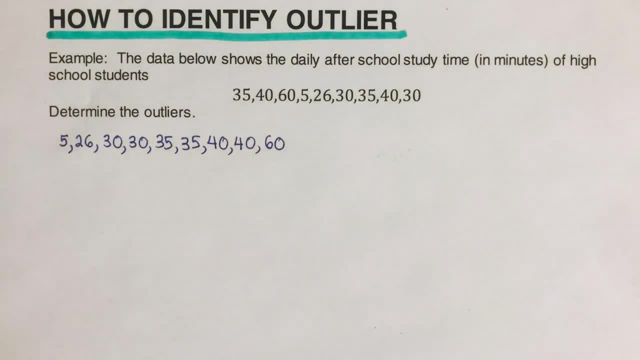 with five, the smallest to the biggest number right there, or that means it's increasing order. Now our next part of this step is to determine the median. In order that we can get the median, we can cover both ends and determine which is the center value or what number is located. 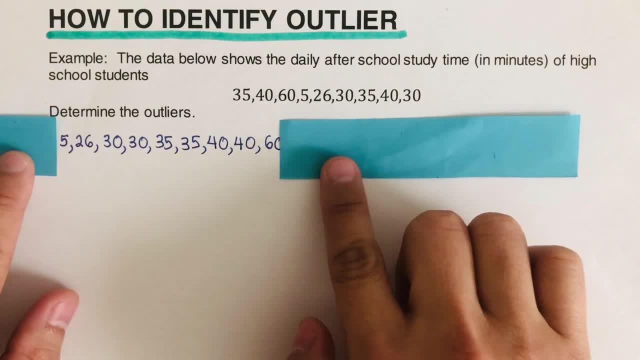 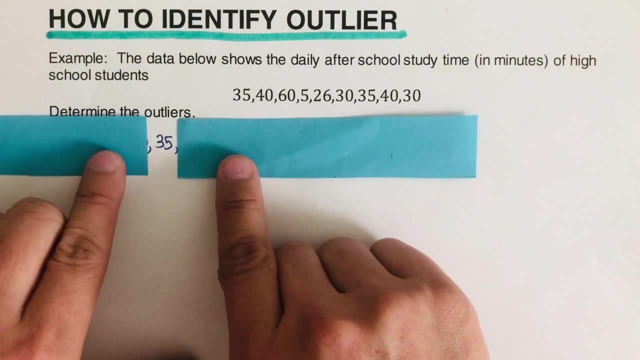 at the center of these set of data. So in this problem, right here, I'm gonna cover both ends, I'm gonna cover the next one, I'm gonna cover the next one, I'm gonna cover the next one. So this value that we have here is the median. 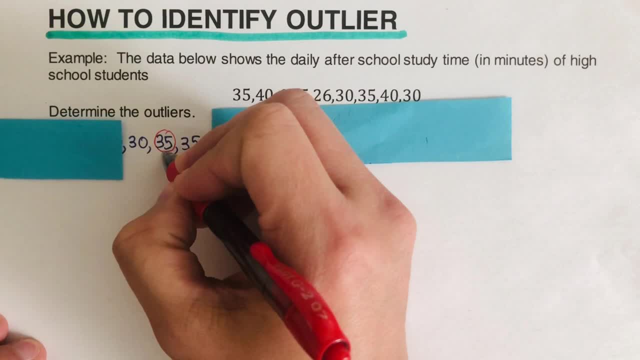 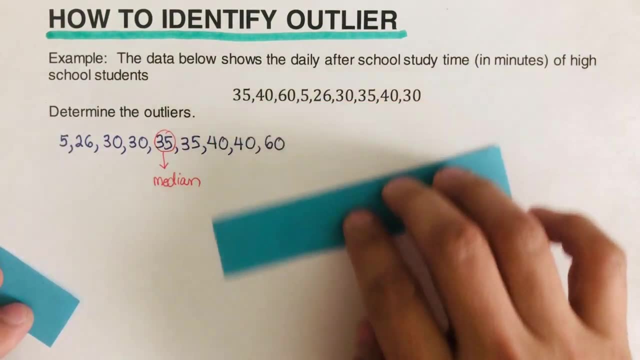 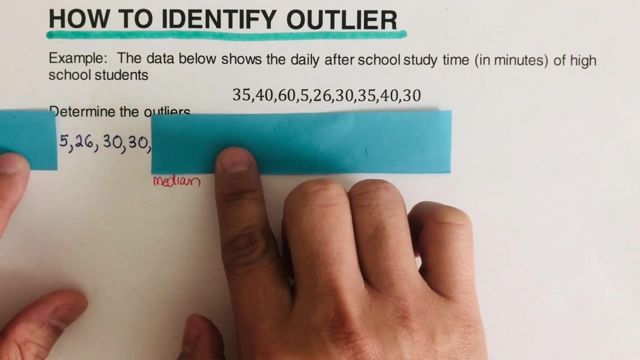 So I can go ahead and circle this. This is our median Now in order to find for Q1, this is already taken, So we're gonna determine the Q1 is actually the median of the lower half. So this is the lower half and this is the upper half. 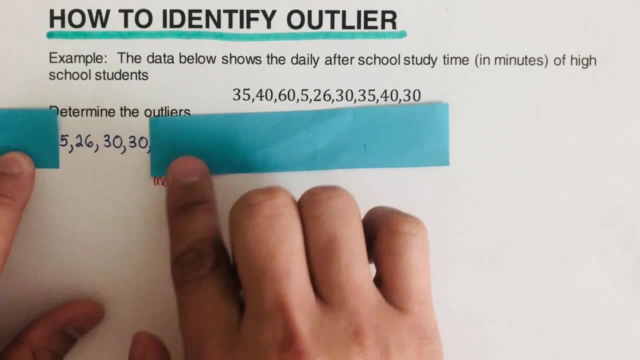 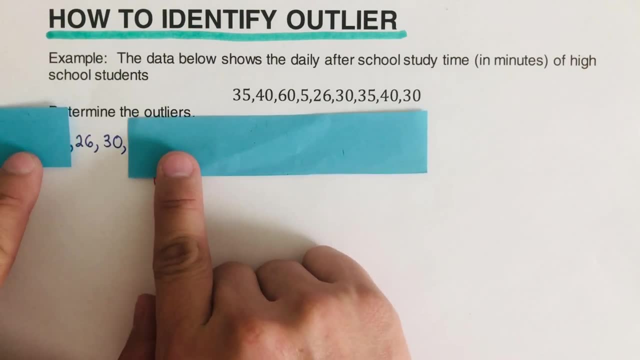 So we're gonna get the median of the lower half. In order to do that, we're supposed to determine the middle of this set of values, So we're gonna cover this, And so we have. we are left with 26 and 30.. 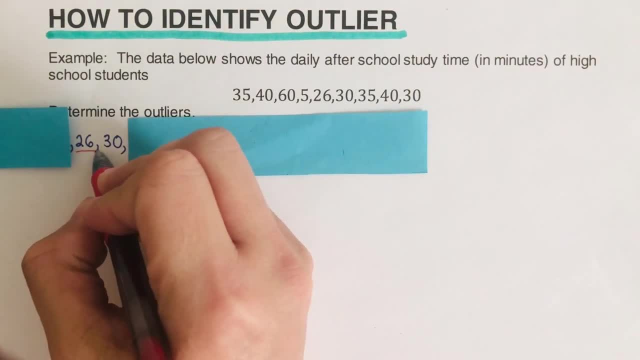 So that means we are supposed to determine the middle value between these two. So it should be somewhere there. So then we can go ahead and add these two together divided by two, so we can get the average. So that would be 26 plus 30 divided by two. 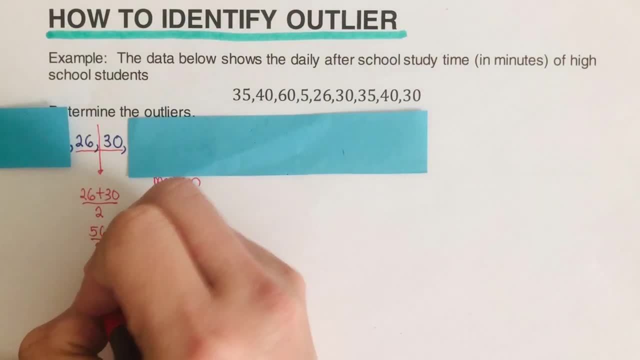 So that is 56 divided by two. So that is 56 divided by two. So that is, 56 divided by two Is gonna be 28.. And then this is our Q1, or our first quartile. I'm just gonna box this. 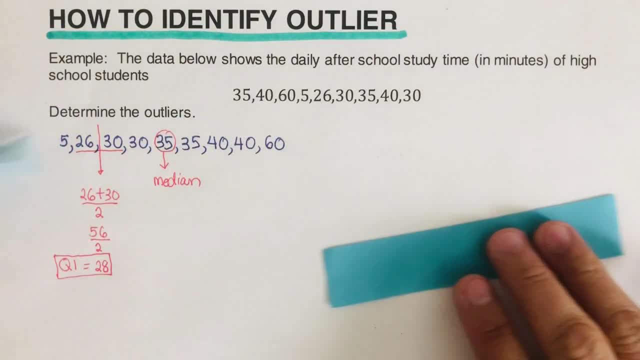 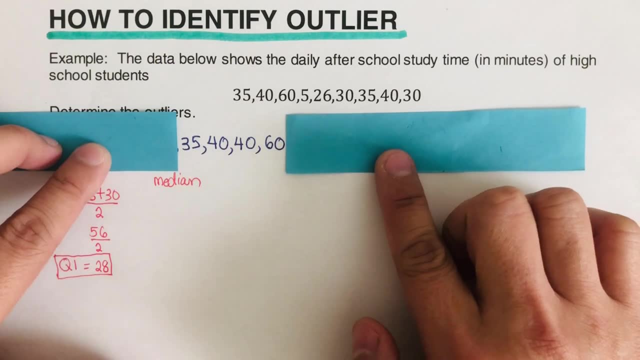 Now we are going to determine the third quartile. So the third quartile is gonna sit on the upper half. So we're gonna take this part right here. So we're gonna cover both ends until we can get the middle. So that part right there. 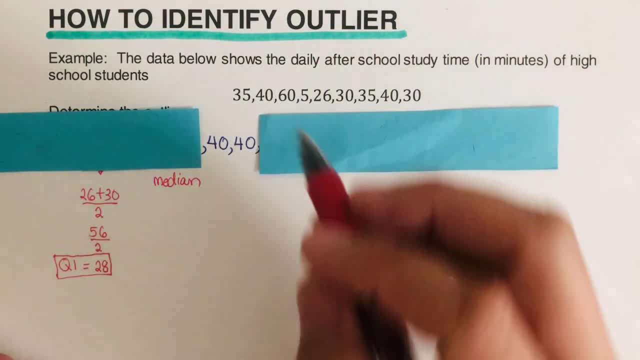 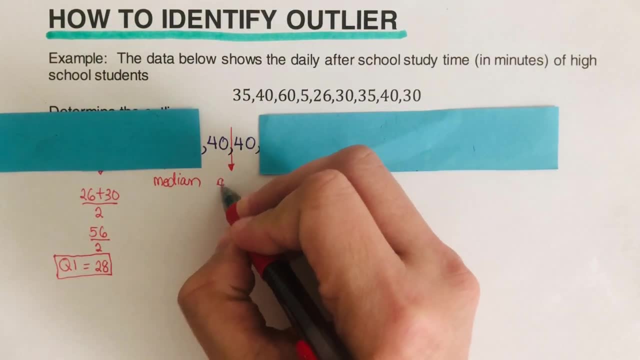 So these two are the middle number for the upper half. So what are we gonna do is we take the middle between these two by getting their average, So we're gonna add both of them, So 40 plus 40 divided by two. 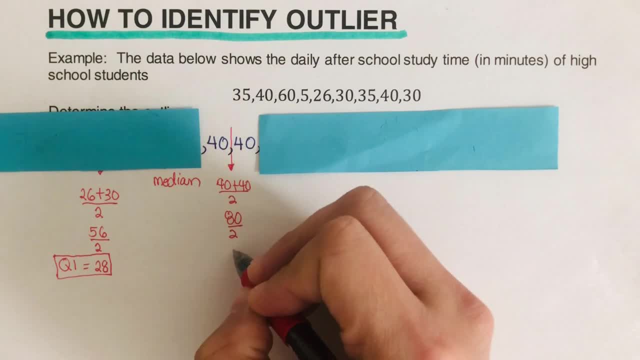 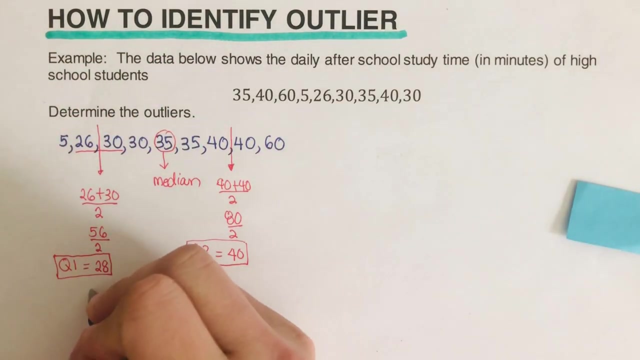 So that's actually 80 divided by two is 40.. So 40 is our Q3 or our third quartile. Now, part of this step is to determine the IQR. So our IQR, then, is equal. to remember, the formula for IQR is Q3 minus Q1. 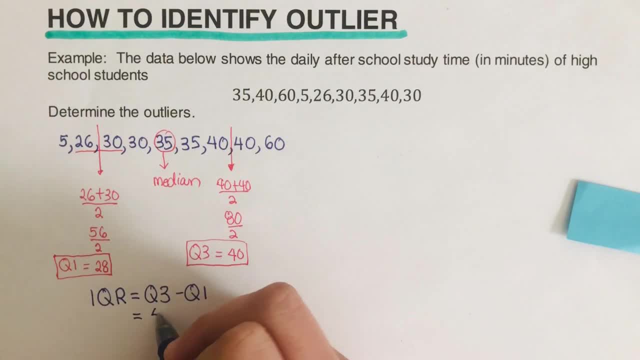 So then from here we can go ahead and plug values in. 40 minus 28 is 12.. So this is our IQR. I'm just gonna put this inside a box. That's our IQR. Now we're ready to determine the outlier for this value. 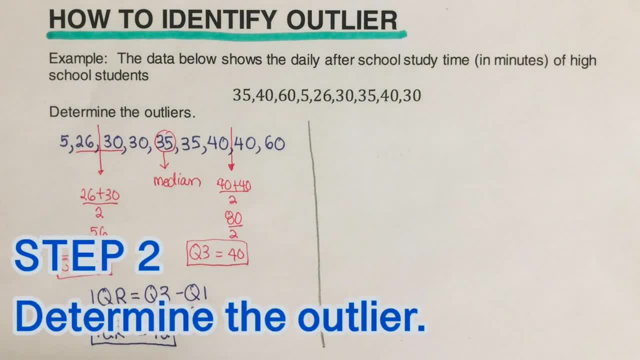 So there are two conditions that we can determine if it's an outlier. remember, If it's way too big, then it's an outlier, If it's way too small, then it's an outlier. So, but then again, we have to come up with an objective method. 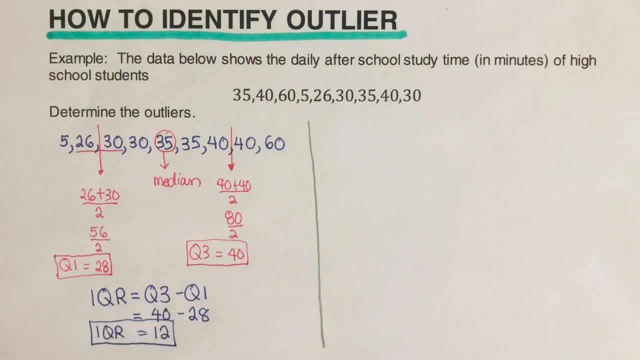 of determining which one is way too big and which one's way too small. So this is the condition in order that we can determine an outlier. So a value in a data set would be an outlier if the value is first condition: if it's greater than Q3 plus the product of 1.5 times IQR. 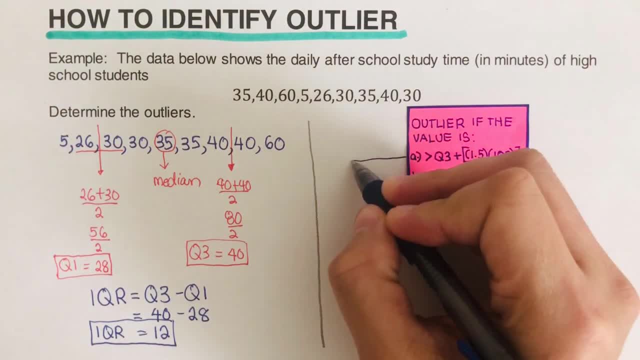 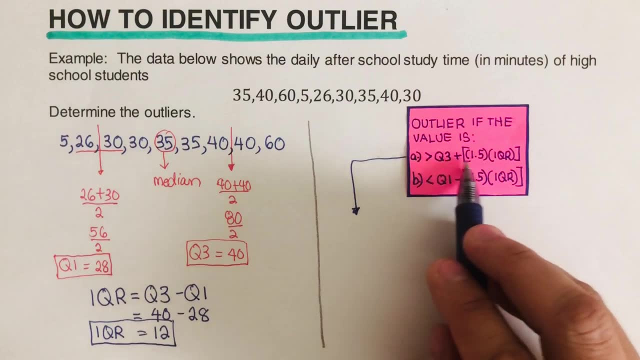 So let's take this first condition right here. So I'm just gonna show the work down here, So using the first one. so anything that is greater than the answer to this would be an outlier. it's way too big. So in this case, right here. 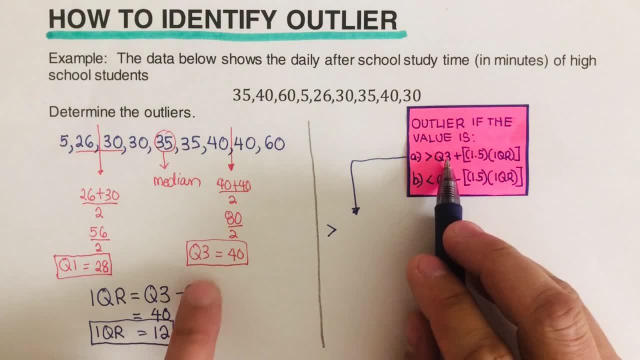 we're gonna have anything that is greater than Q3 is 40. So I'm gonna write 40 plus and then that's a bracket right there, 1.5 times. our IQR is 12. So I'm gonna write 12 here. 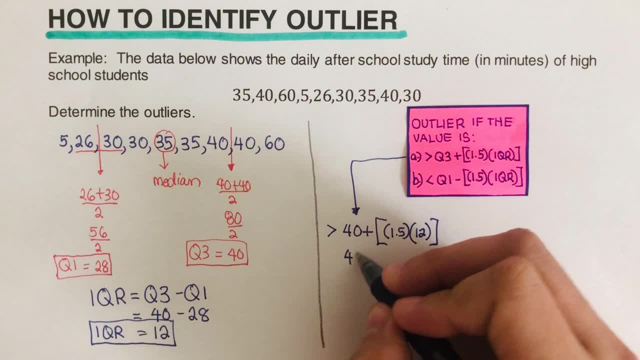 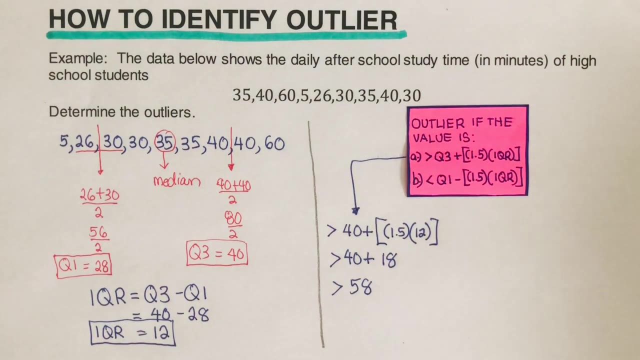 and then I'll just do the arithmetic for this. So that would be 40 plus 1.5 times 12 is 18.. So that's gonna be 18.. So anything greater than 58 is an outlier. So in this problem that we have here, 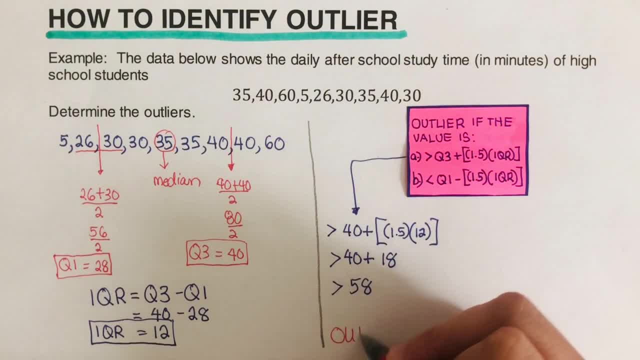 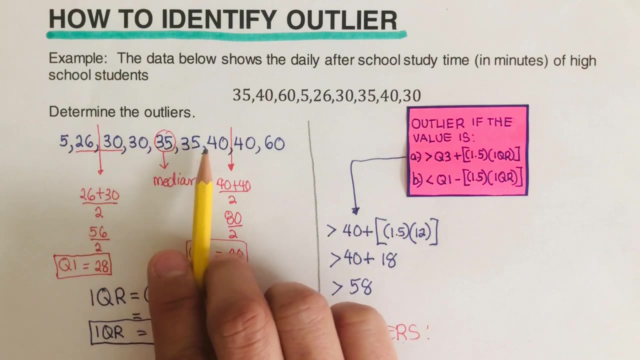 we can therefore say that these are our outliers. That means they are either way too big or way too small, So let's start with anything that is greater than 58.. So we go back to the set of numbers we have here. Any number that is greater than 58 is an outlier. 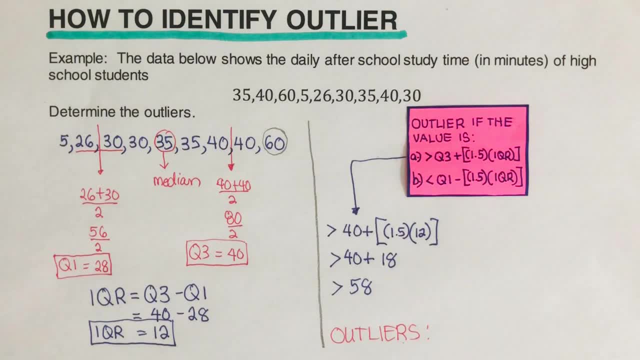 60 is an outlier. it's way too big, And we can justify this because 60 is way far from 40. So that's way off, that's way too big. So the first outlier then is 60, because 60 is greater than 58.. 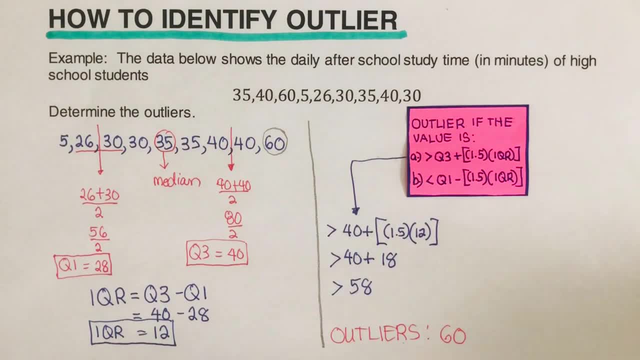 So I'm just gonna write 60 here. Now let's determine the other outlier, which is way too small. So let's see what number is considered an outlier. that's again, it's way too small. So we're going to use the second condition that we have here. 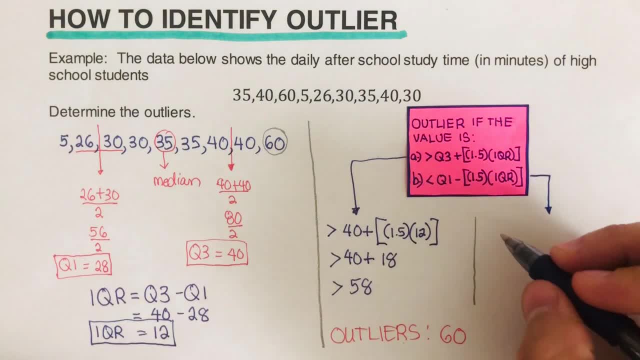 So in the second condition we say that anything that is less than Q3, our Q1 is 28.. So I'm gonna write: 28 minus that's 1.5 times, our IQR is 12.. So then we go ahead and do the math here. 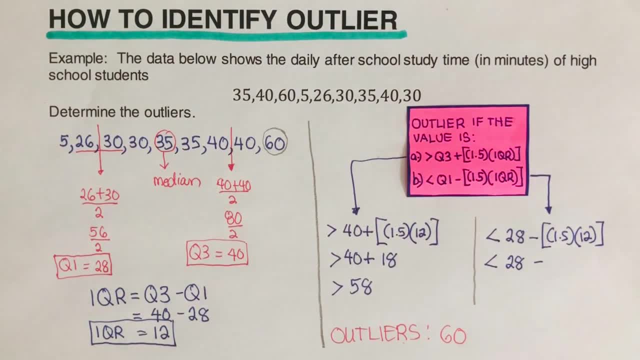 So anything less than 28 minus 1.5 times 12 is 18.. So then we can go ahead and say anything less than 10 is an outlier. So we go to the set of data that we have here: Anything less than 10.. 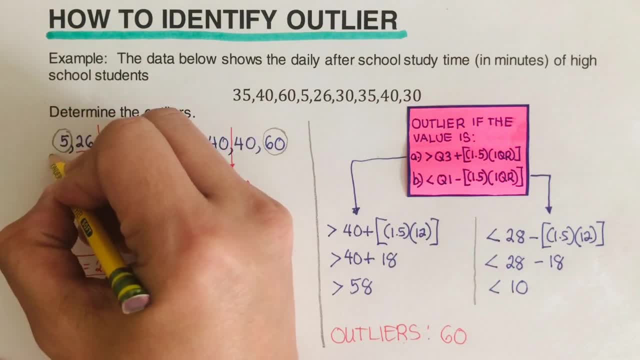 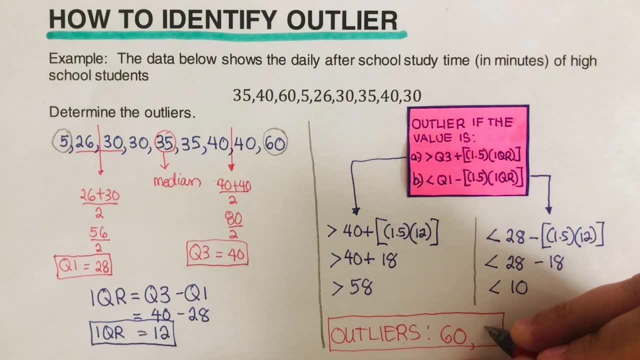 So five is less than 10.. So this is an outlier. So then we can add five as one of the outlier, because again, five is way too small. Again it's less than 10.. So it's an outlier. So these two are the values that are considered outliers. 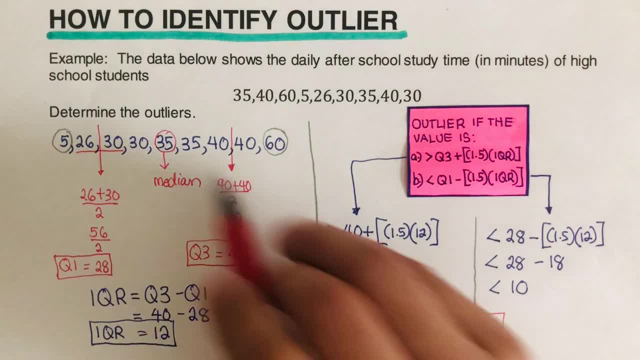 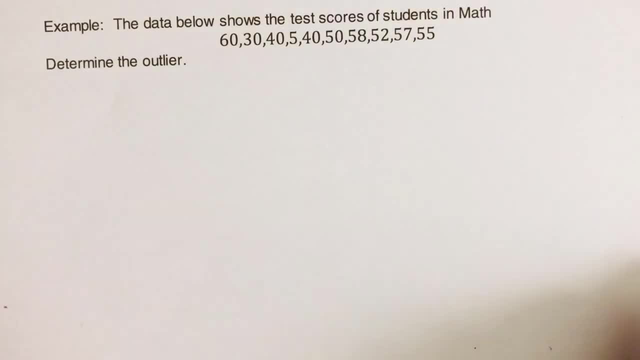 60 is way too big than the rest of them. Five is way too small compared to the rest of them. this time i would encourage you to pause this video and try this problem out on your own and, when you're done, and pause it and check your answer. 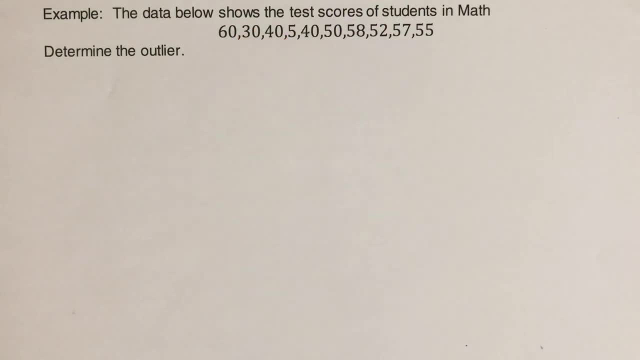 okay, so we go over the problem here again. we are given the data that we have here shows the test score of students in math, so these are their scores. now we determine what are which of these numbers that we have here are considered an outlier. again, the first step is to arrange these. 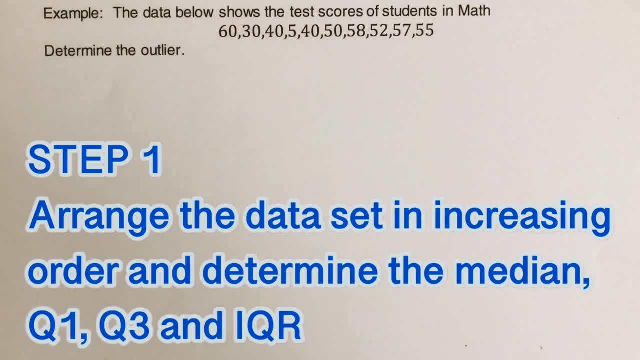 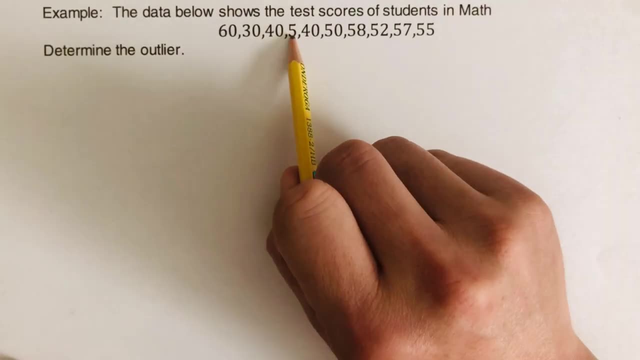 values from smallest to biggest, and then we determine the median, and we determine the median q1- first quartile, q3- third quartile, and the iqr. so in this problem that we have here, we determine the lowest value was 5 and the highest value is 60, so then we can go ahead. 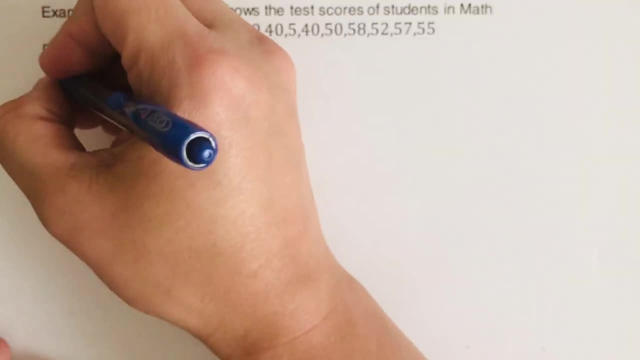 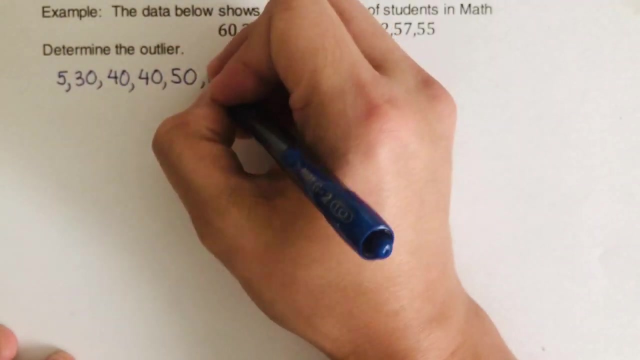 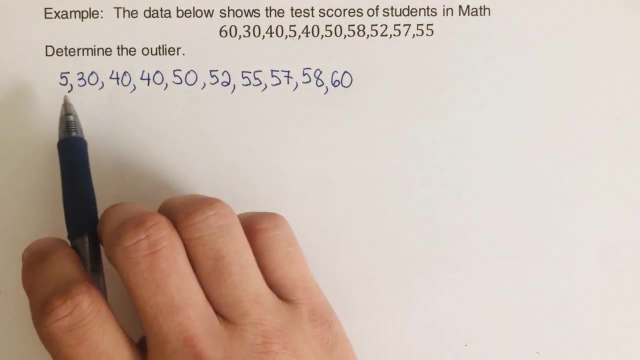 and arrange them in order, starting with 5. so i'm just gonna write 5. so okay, so i have arranged the values from smallest to the biggest value that we have here. part of the first step is to determine the median. again, we can determine the median by getting the. 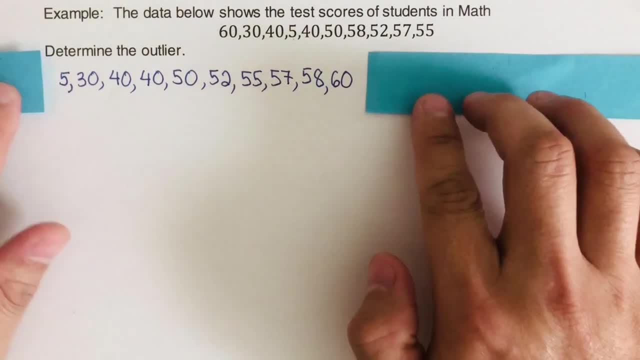 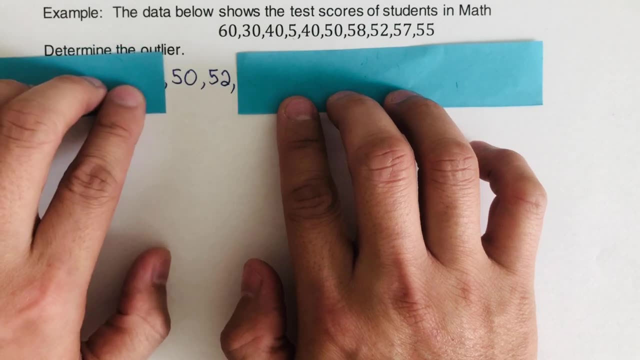 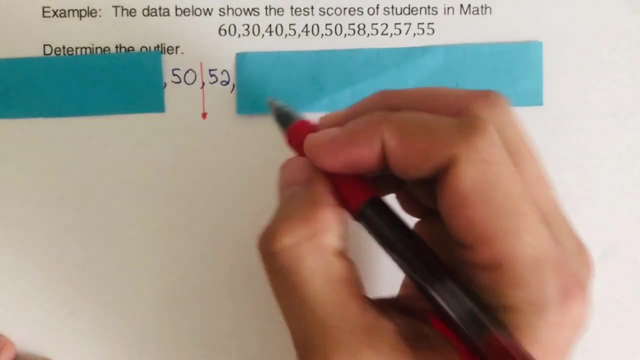 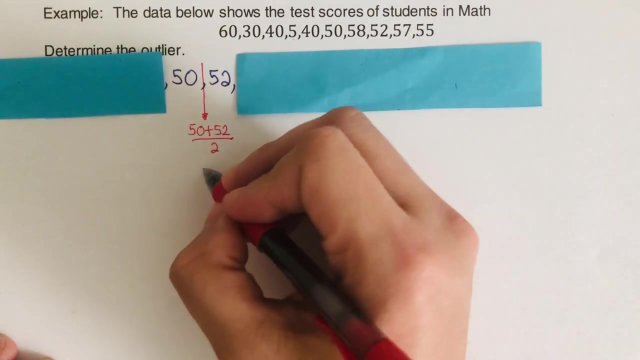 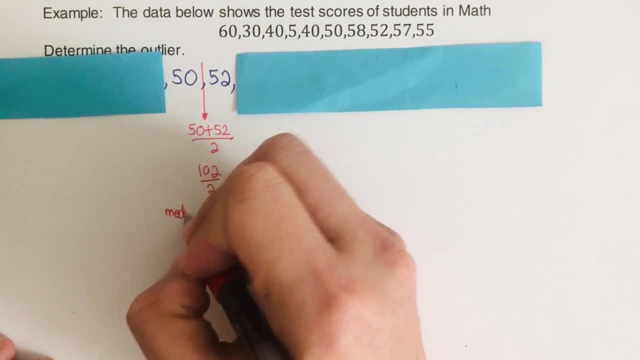 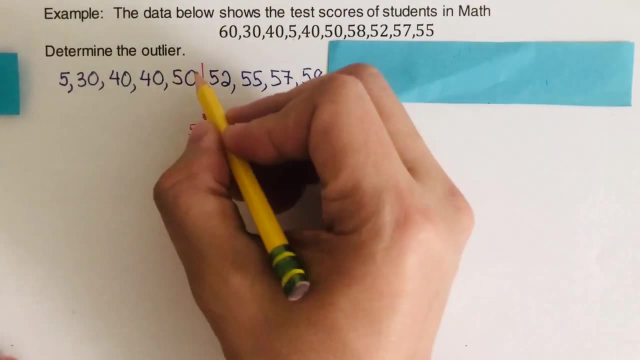 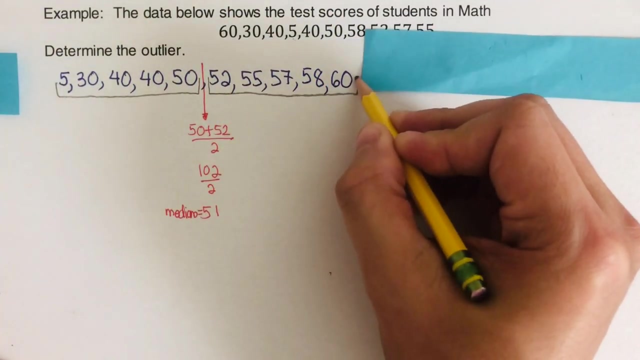 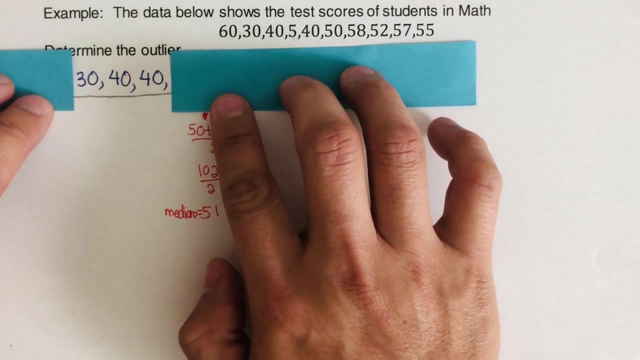 our median. so i'm just gonna label this as median. now let's find the median of the lower half. so 50 is not the median. so that means this is our lower half and this is our upper half. so we're going to determine the median of the lower half. again, we do the same thing: cover both ends, cover both ends. 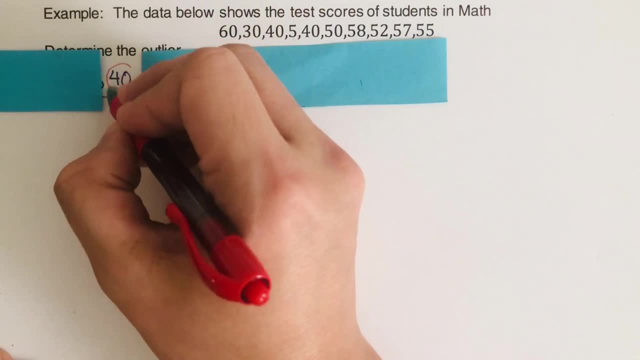 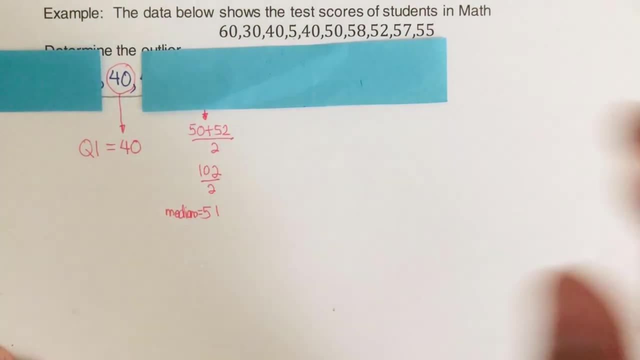 until we can get the middle. so our q1 is 40. so i'm just gonna label this as the q1, which is equal to 40, and then we determine the q3 from the upper half, which is the median of the lower half. so we're 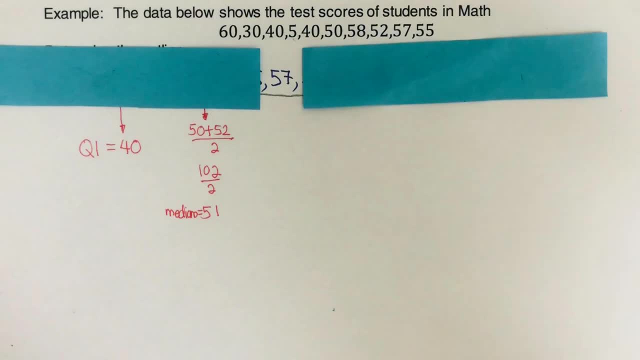 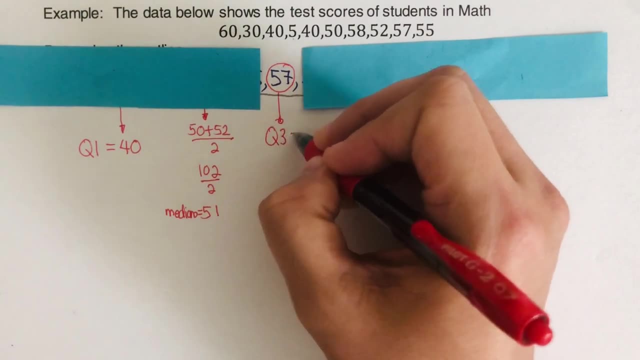 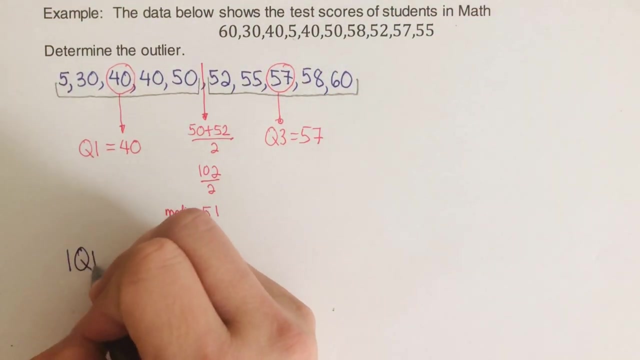 going to determine the median of the upper half. so we cover both ends, cover both ends. so it's 57, is our third quartile, or q3, and then again that's 57. so then our next step is to determine our iqr. again, the formula for iqr is q3 minus q1, so then our q3 is 57, 57 minus the q1 is 40. 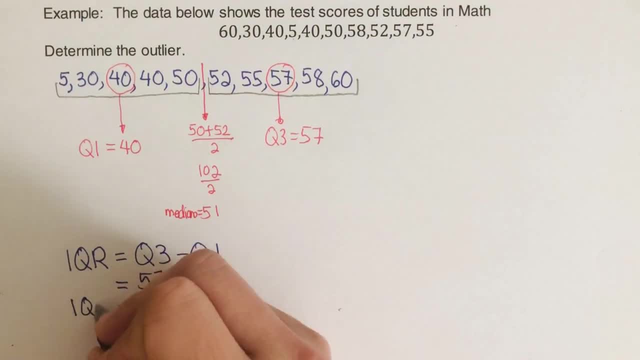 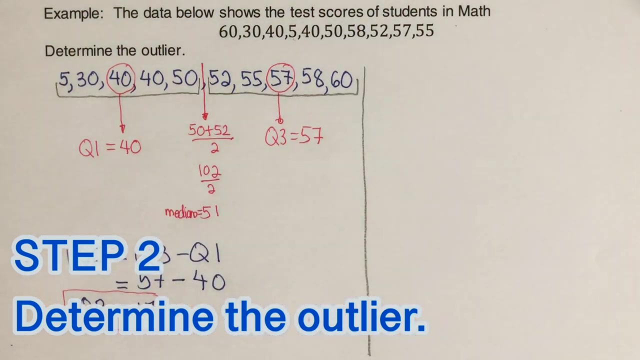 so that would be 17. so that is our interquartile range. so i'm just gonna box this. now we are ready to determine what which of these values that we have here, in increasing order, which of these values are considered outlier. again, outlier are numbers that are way too small or way too big than the rest. 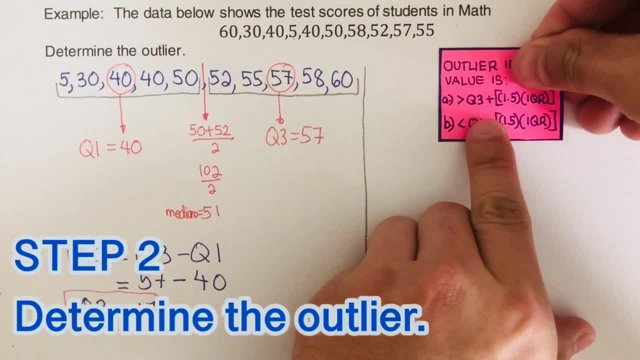 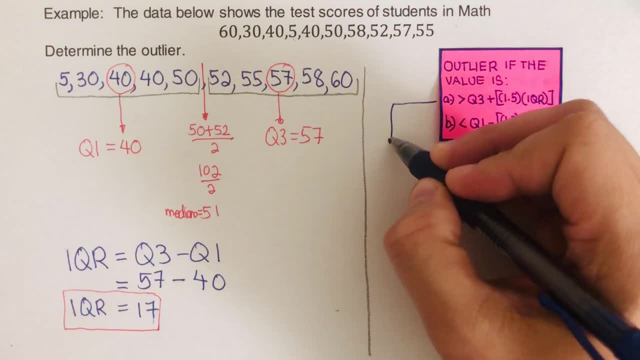 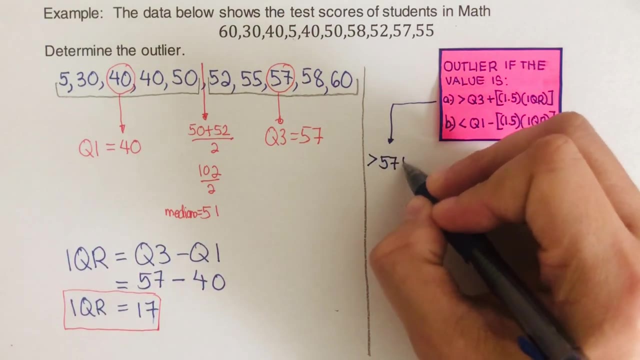 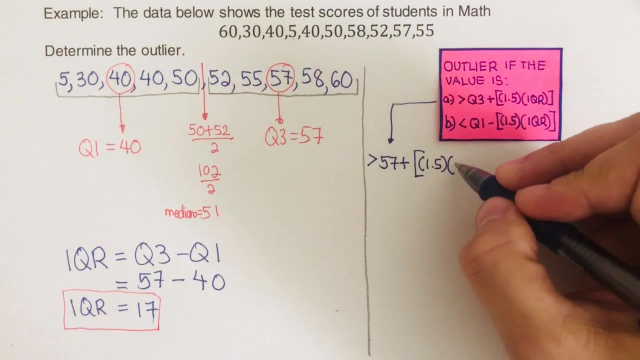 of them. so let's go over these conditions that we have here. so let's start first with the one that is way too big. so that is anything that is bigger than the answer to um. that's gonna be q3. our q3 is 57 plus our um, that's 1.5 times. our iqr is 17, so i'm just gonna write 17 there, and so this becomes: 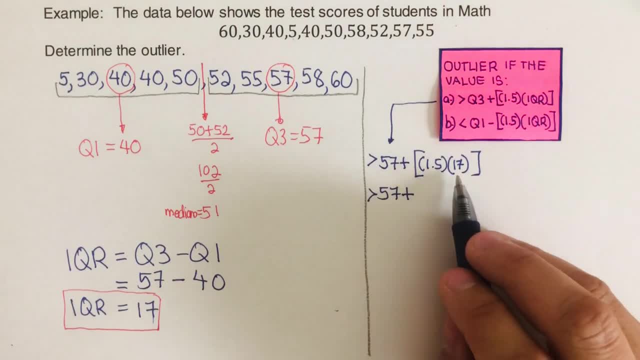 57 plus 1.5 times 17 is 25.5. so then we add them up together that would equal to 82.5. so anything that is bigger than 82.5 are considered outliers. i'm just gonna- we're gonna- list them all down here, so that's outlier, okay. so let's look at the values that. 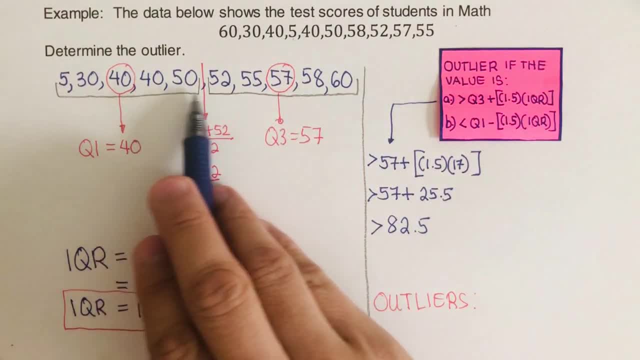 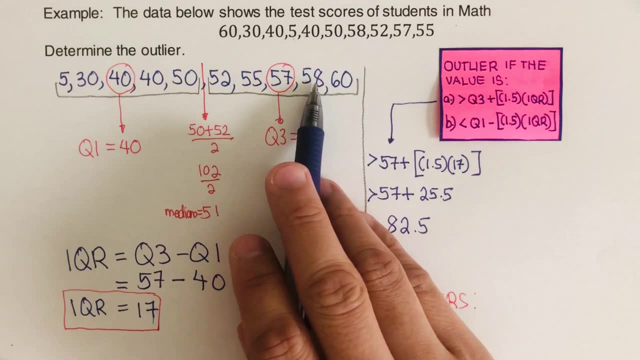 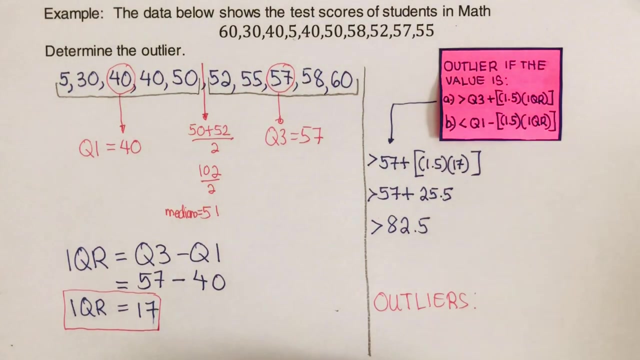 we have. is there anything greater than 82.5? so nothing is greater than 82.5. that makes sense. 60 is not an outlier here, because 60 is closer to 58 and 57, so they're pretty much like um, closer to each other. now let's see the other condition: that we have anything that is lower.